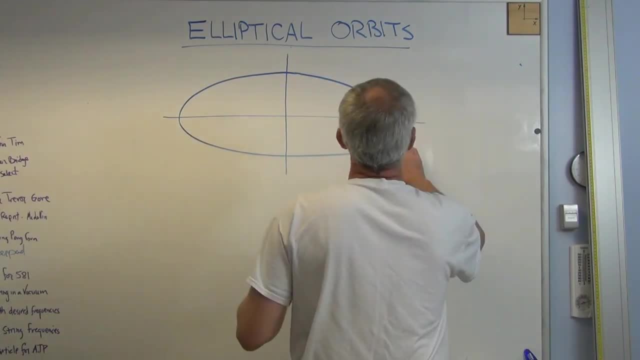 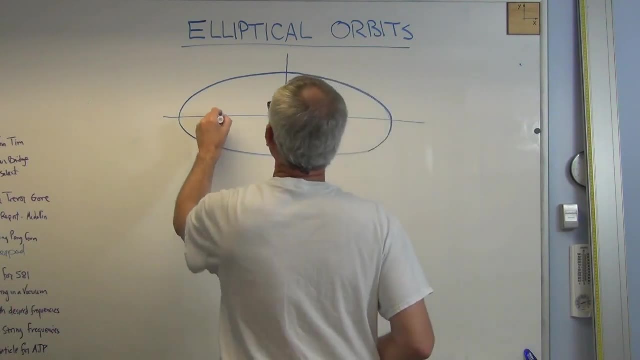 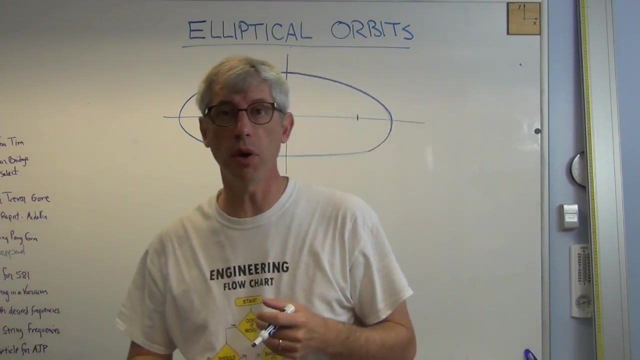 up a little bit There. There, that's slightly less terrible. Anyway, how do you make an ellipse? by the way, You guys know, There's two points in there. Each point is called a focus And the plural of focus in English is foci. Nobody uses that word much, but there's. 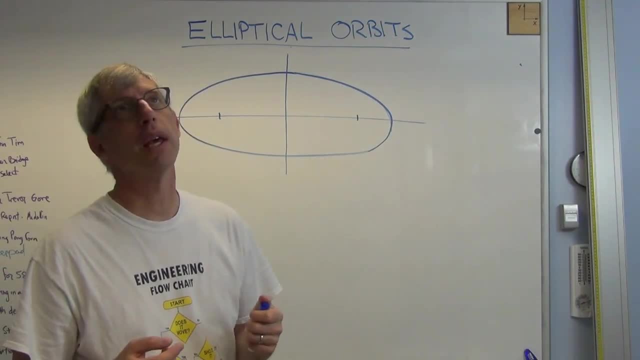 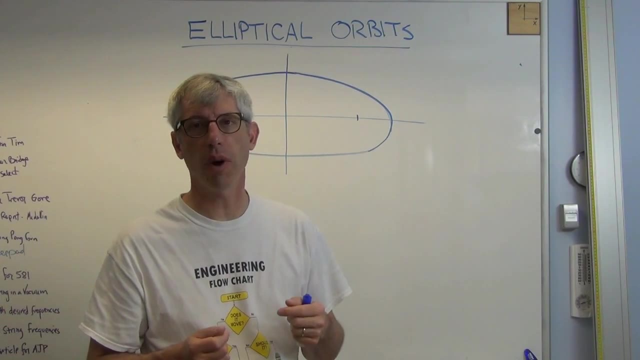 no such word as focuses. Well, he focuses the camera. Yeah, that's a word, But to describe two foci, Focuses is not the right plural. It's called foci And what these are if you draw a line. 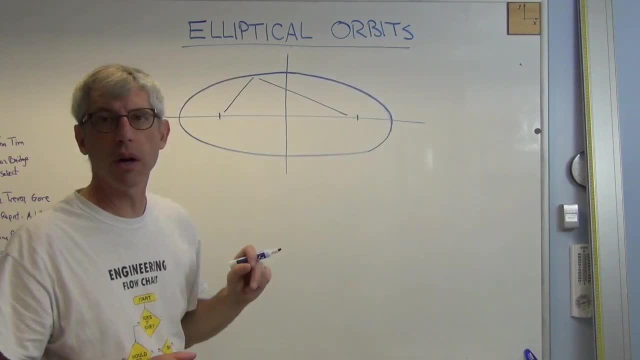 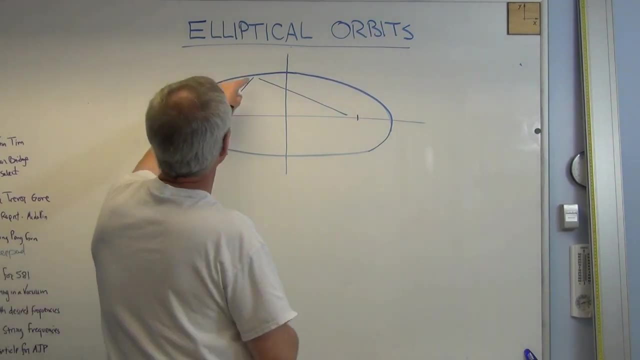 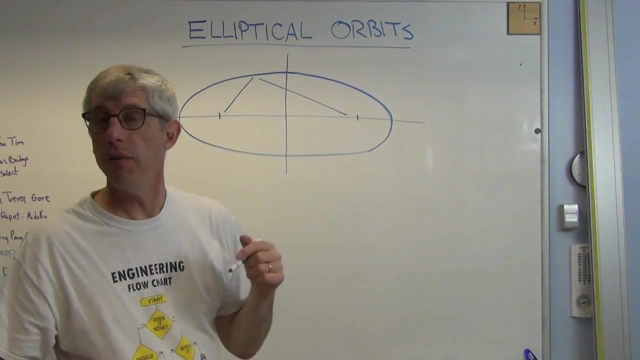 from one focus to the other and touching any part of the ellipse, the length of that line plus that line is the same, no matter where you are on the ellipse. So if I take this point and I can rotate this all the way around, some of those two lengths wouldn't change. 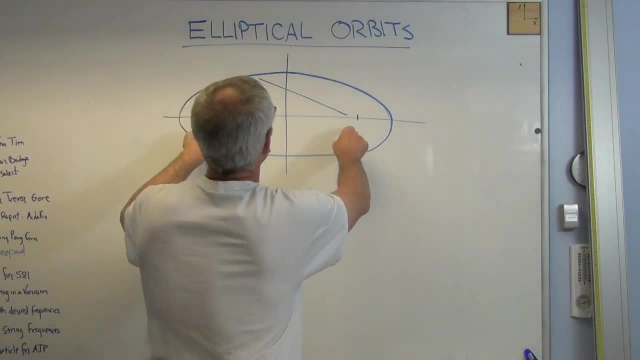 In fact, if you want to make an ellipse mechanically, you can put two nails in a board, tie a string between them and make sure the string is loose and then just put a pencil on the string. hold the pencil tight. it'll trace out an ellipse. That's how you make an ellipse. That's. 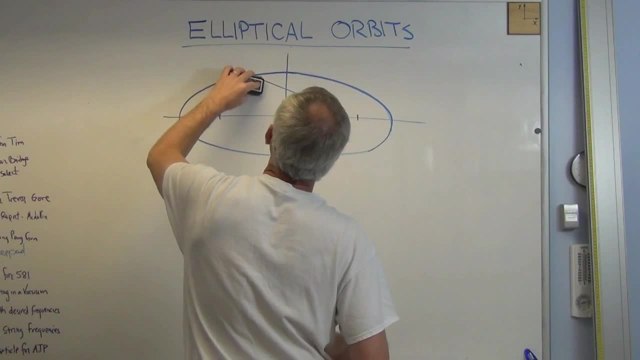 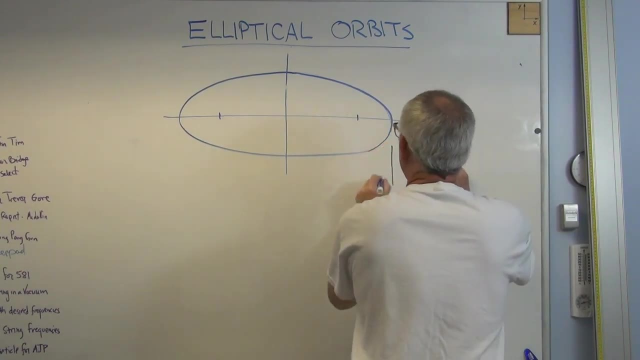 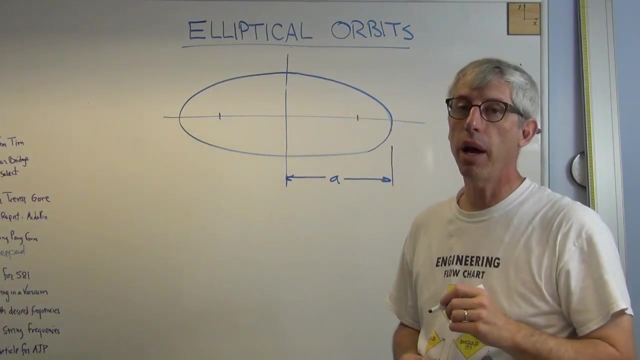 what the equation for an ellipse is really telling you. Alright. so let's get to the terminology here. Half the width of the long length. here it's almost always called A. by the way, not sure why that is called a semi-major axis, Not. 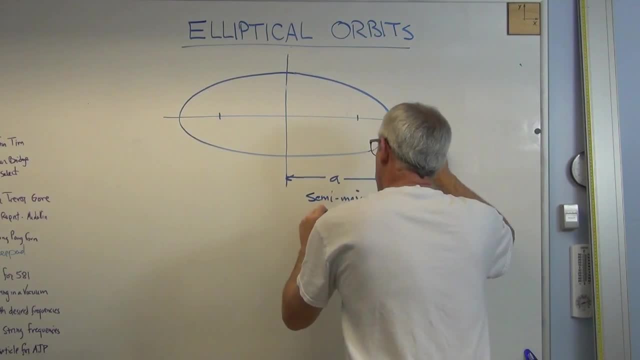 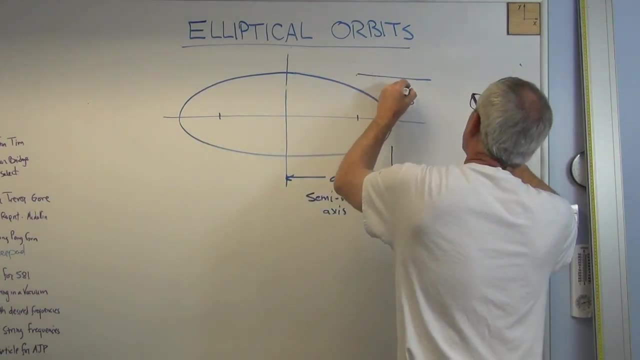 the word I would use, probably, but it works. That's the semi-major axis. That's half the long distance This up here. B is the semi-minor axis. Why did they name it that? I don't know. 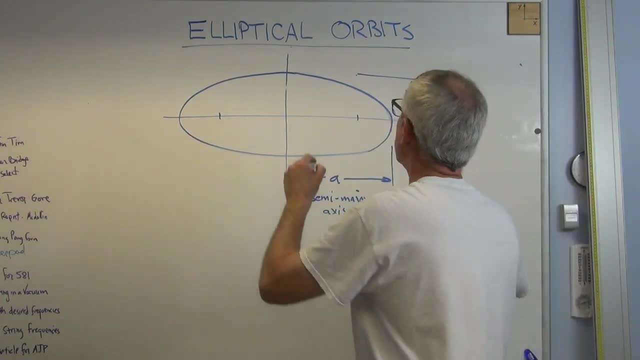 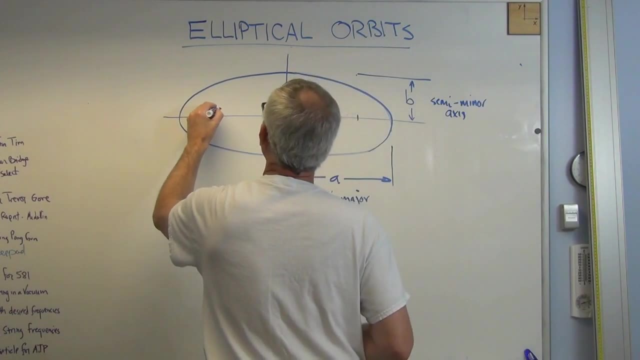 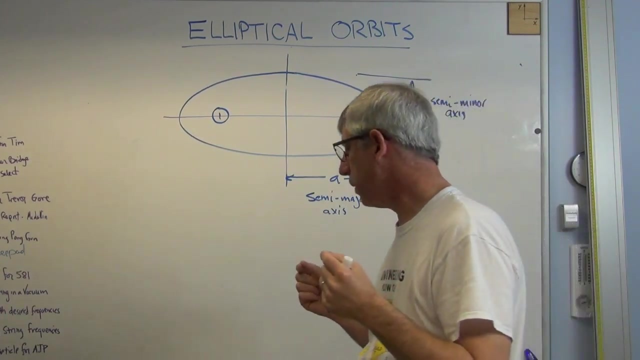 Why do mathematicians do anything? So let's see, we've got that, The other distances we've got here. let's put a planet here, Let's put the Earth right there. perhaps When one body orbits another one, the thing 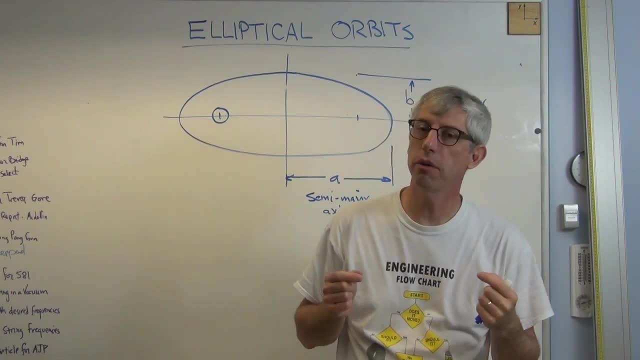 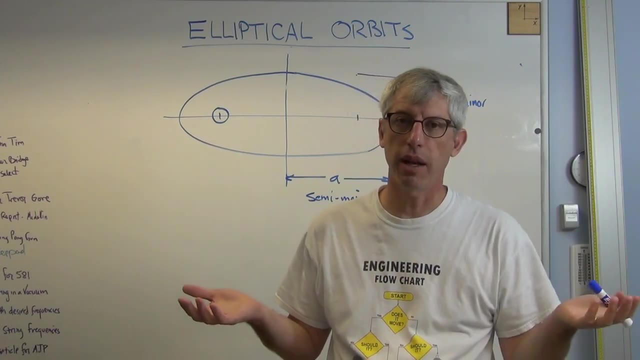 that stays at. the focus is actually their mutual center of gravity. But let's think about this a second. The Earth weighs something like 10 to the 24 kilograms, and a satellite weighs like 10 to the 3, maybe 10 to the 4 kilograms. The mass of the Earth is just gargantuan. compared to the mass of the satellite. So in theory, yeah, the Earth moves a little bit, but it's a tiny, tiny number and completely non-existent. Now, when a planet orbits the Sun, now the Earth is massive, but it's not massive compared. 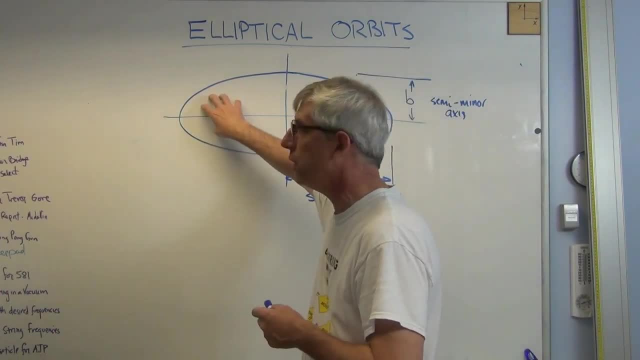 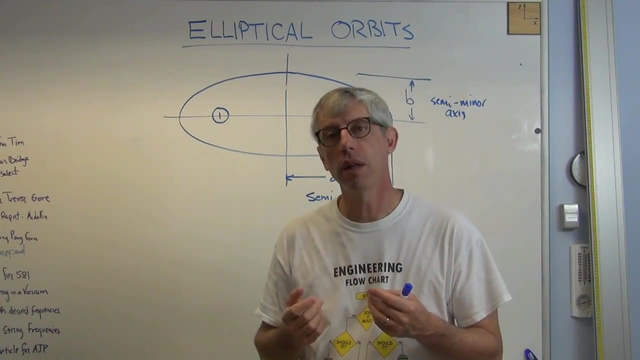 to the Sun. The Sun is many orders of magnitude larger in mass than the Earth. So while the Sun orbits the Earth, does the Sun oscillate just a little? Yeah, it does. But if we treat the center of the Sun as being one focus of the ellipse that describes the orbit of the 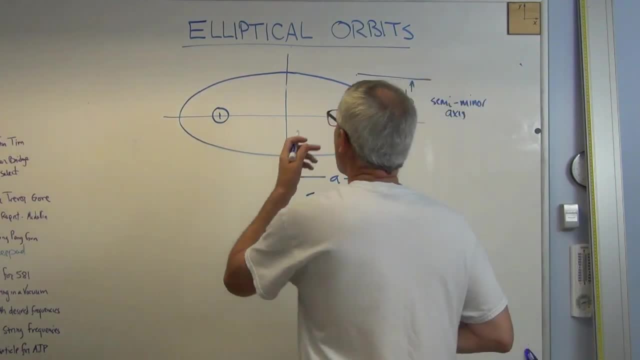 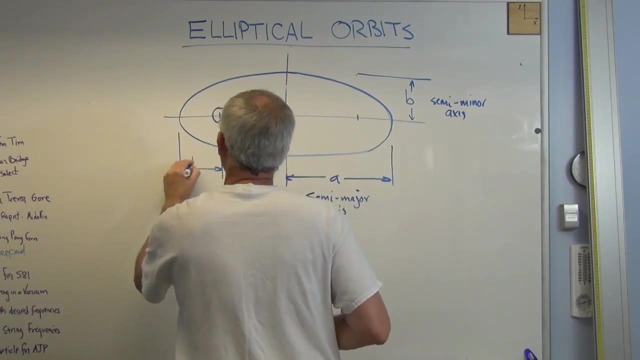 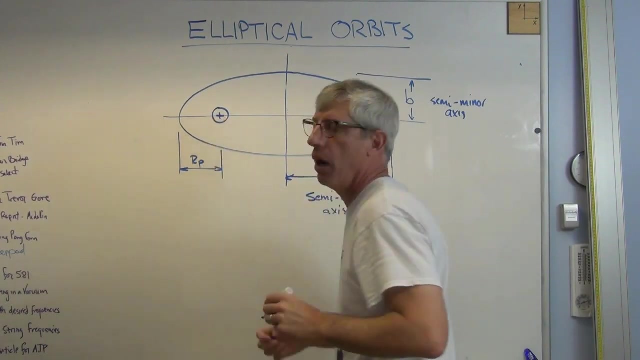 Earth around the Sun. you still pretty much get the right answer. So there's a funny number we need here The distance, That thing right there, The point of closest approach from the satellite to the Earth. I like this better Satellite to the Earth That's called the perigee, And 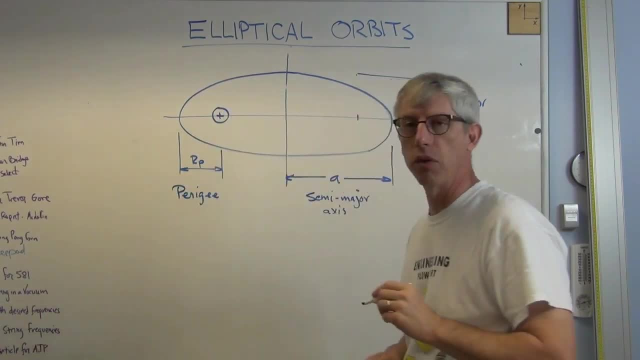 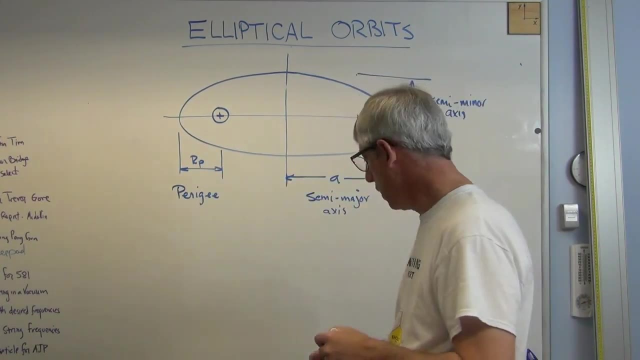 this is, I don't know, I think maybe a Greek word or based on Greek. Alright, Well, there's a number for the closest approach. There must be a number for the farthest approach. Now, we're not going to use this B number here, so I'm going to erase that to get it out of. 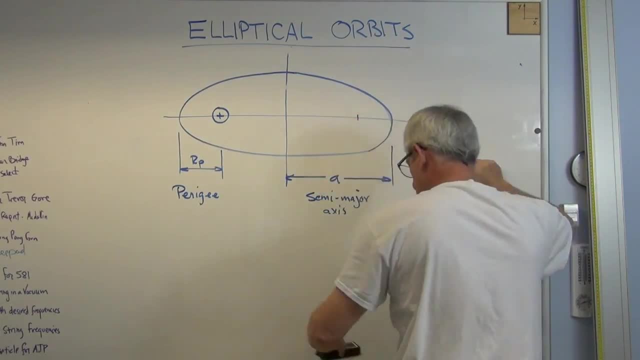 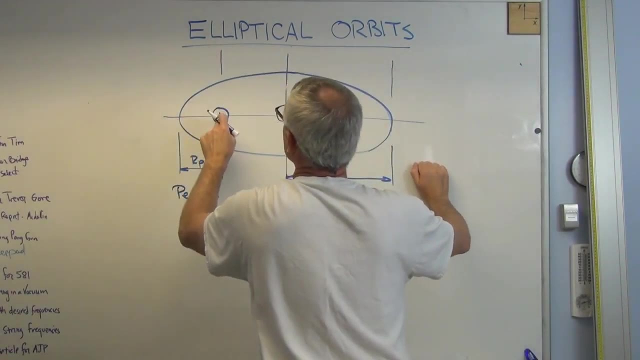 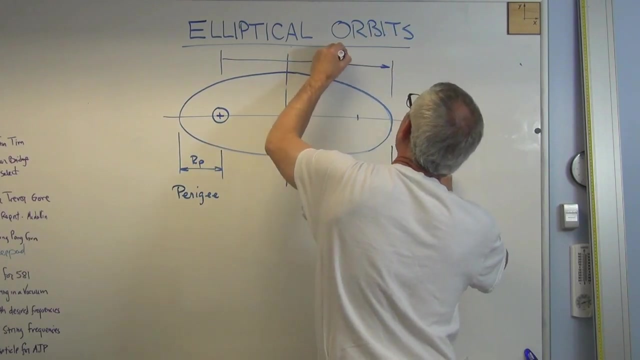 the way It's there, You'll see it, But we don't need it for this calculation, okay, And I want to keep things as tidy as I can. So this distance right there from the center of the Earth to this farthest approach, we'll call that RA And that's called the apogee. Okay, Again. 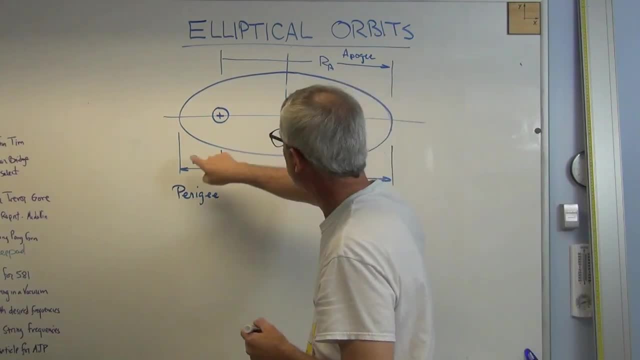 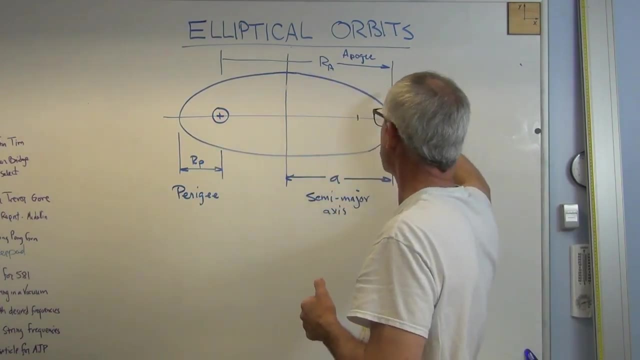 I think it's a Greek word. Perigee is the closest approach, measured from the path of the orbit to the center of the Earth, not the surface. And then the apogee is from the center of the Earth to the farthest distance from the Earth. If this number after this, 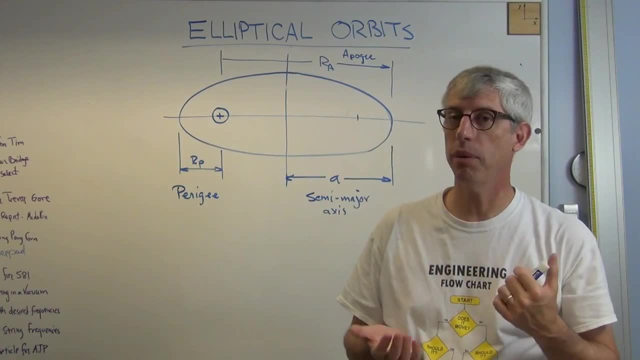 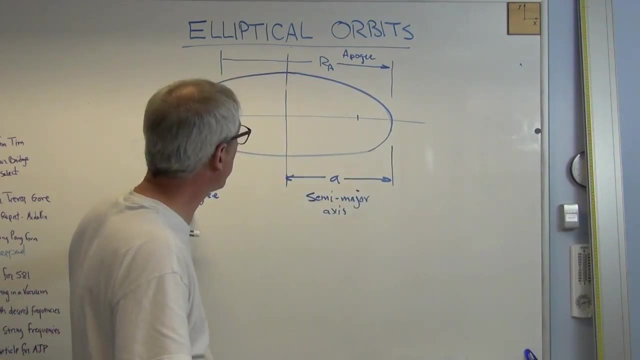 word actually changes depending on what you're orbiting. again, I probably wouldn't have picked it this way, but that's how it is. If you are orbiting the Sun, this is called the perihelion and that is the aphelion. If you are orbiting the Moon, that becomes the perilune and the 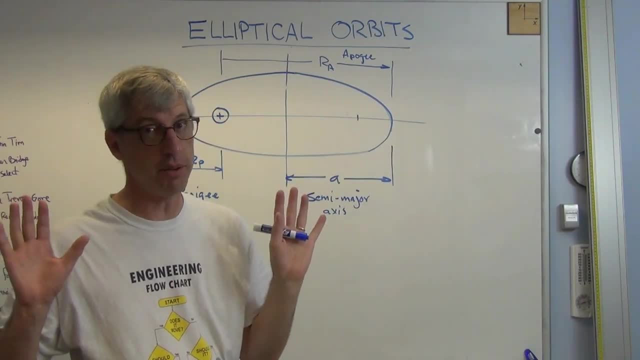 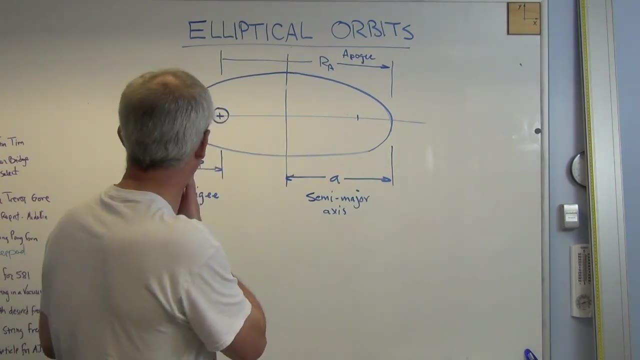 apolune. Okay, Again, I'm just reporting the news here. This is, this is what's happening, This is what it's called. So, since we're we're saying that this is the Earth, we'll call that perigee and apogee. So let's see, we've got perigee, apogee, semi-major axis. 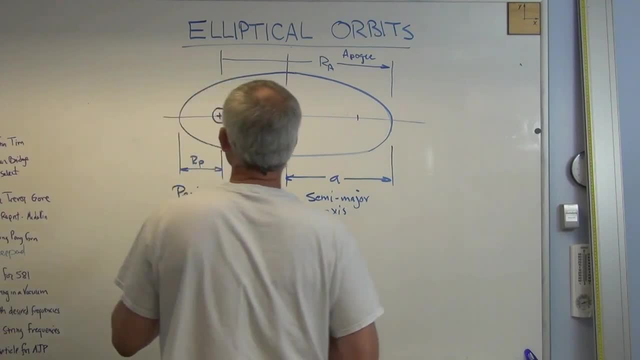 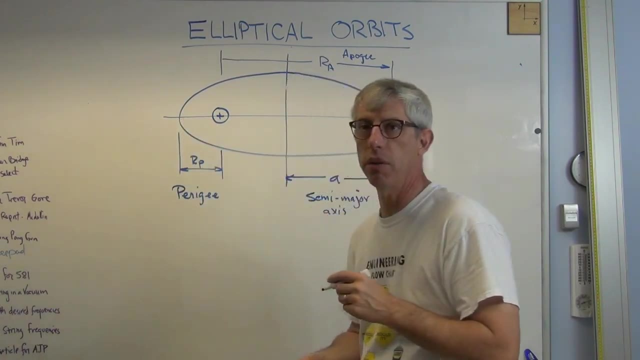 That's all the stuff we're going to need here. One more thing we'll need, actually We need to know one more number. Either we either need that number directly or we need the height of the orbit above the Earth. one of the two We can extract one from the other, So let's. 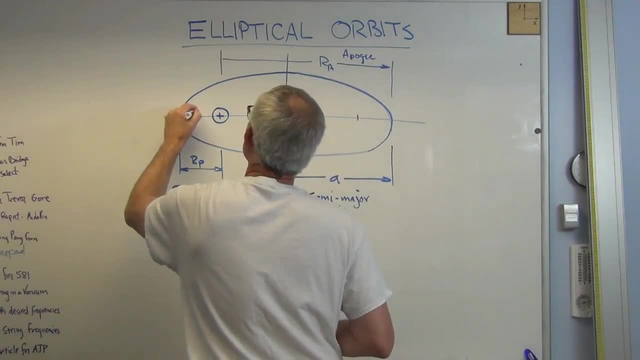 say that this closest approach- and I'll call this H- It's 400 kilometers. Now, that's measured from the surface of the Earth. Okay, And we do it that way because, you know, as we watch the satellites go overhead, we want to know. 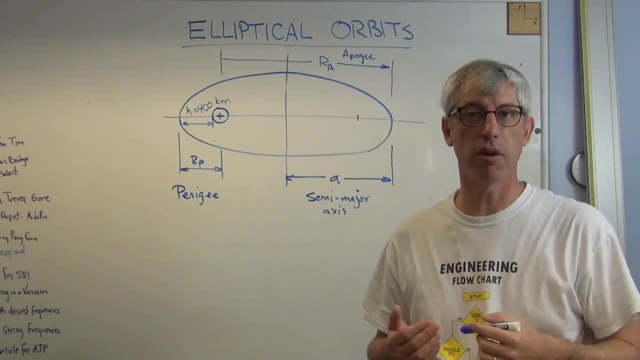 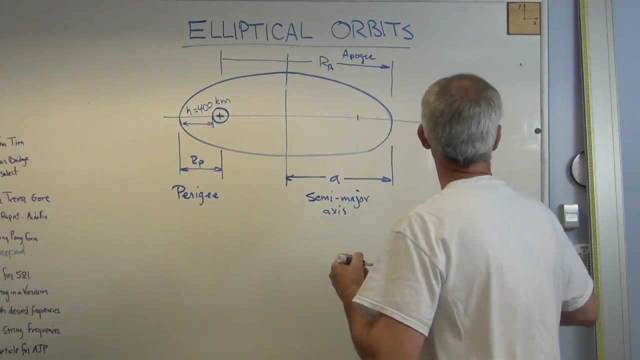 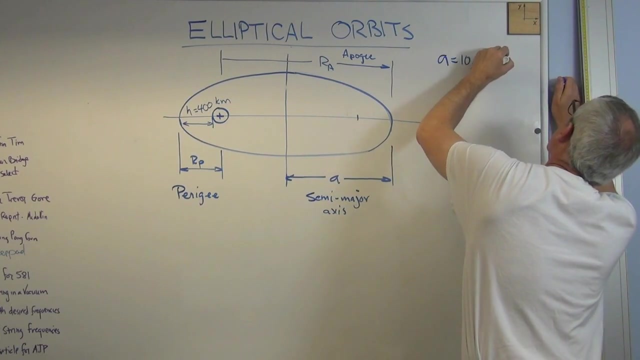 how high above us they are. I don't care how far it is from the center of the Earth, I want to know how far above, But it's- 400 kilometers from the surface of the Earth is generally low Earth orbit. Alright, so let's see If A let's make this big, but not crazy big. 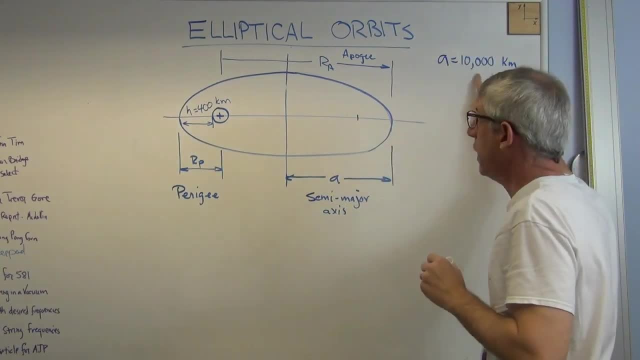 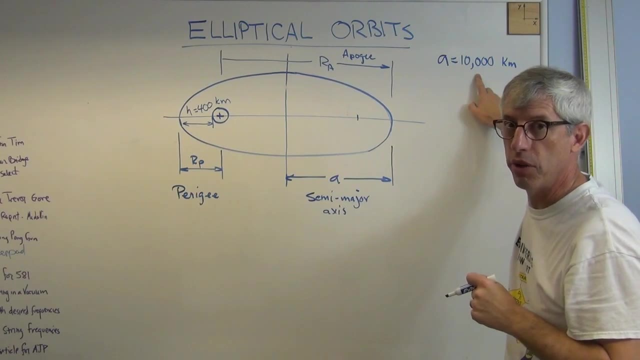 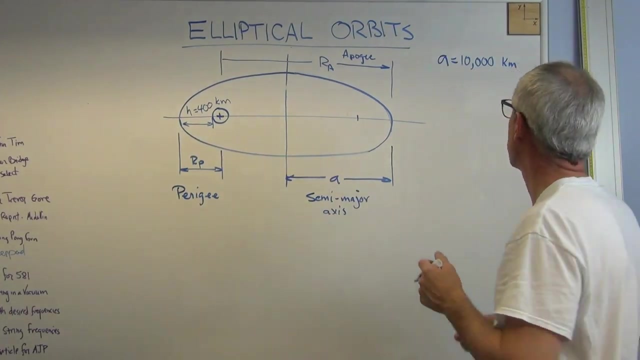 I use 10,000 kilometers. Okay, If A can get really, really, really big. if, like, if you look at the orbit of Halley's Comet, it's measured in astronomical units, where an astronomical unit is the distance from the Earth to the Sun, It'll be millions, billions of kilometers. Okay, H we've already. 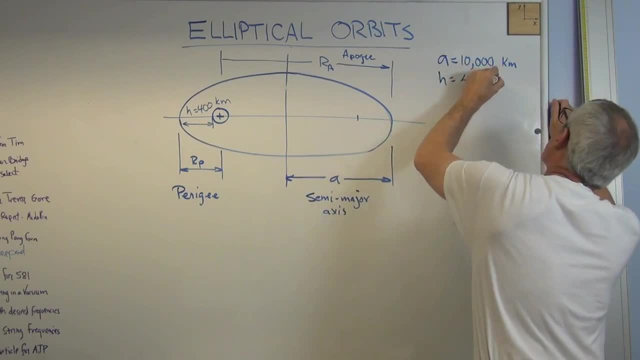 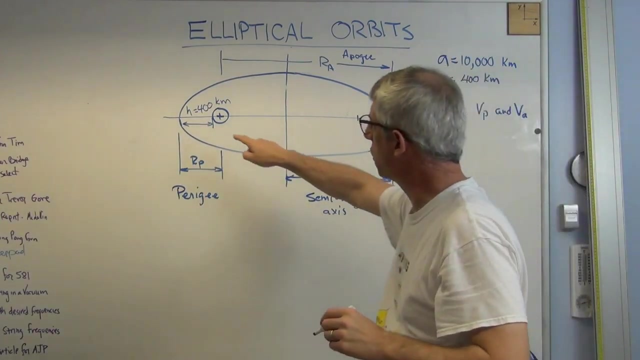 decided is 400 kilometers. Alright, anything else we need to know here? I think that's it. So let's find V, V, V, V, V at the perigee, V at the apogee. Now, if this was a circular orbit, we found out last time that v of a. 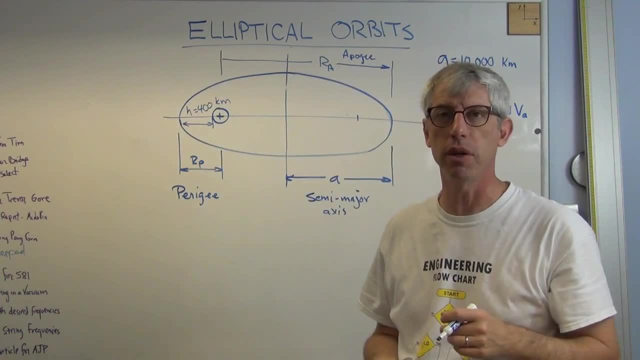 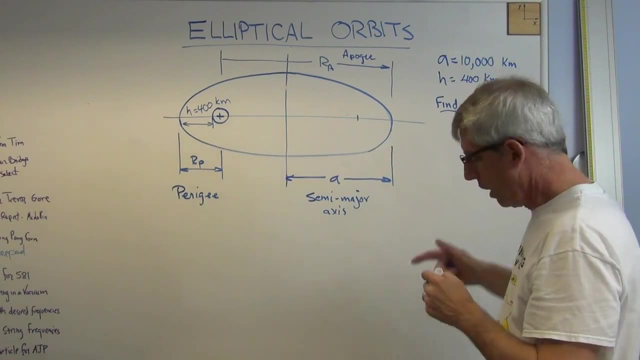 circular orbit is about 7.7 kilometers per second, 7700 meters per second. Well, if we do this right, that number ought to be more than that. and be less than that, Because what happens is during a cyclical orbit or an elliptical orbit, as the orbiting body passes. 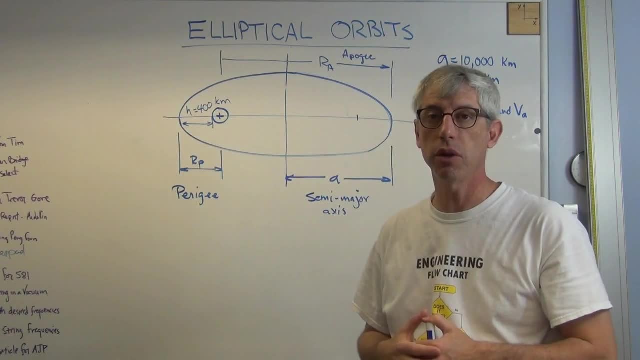 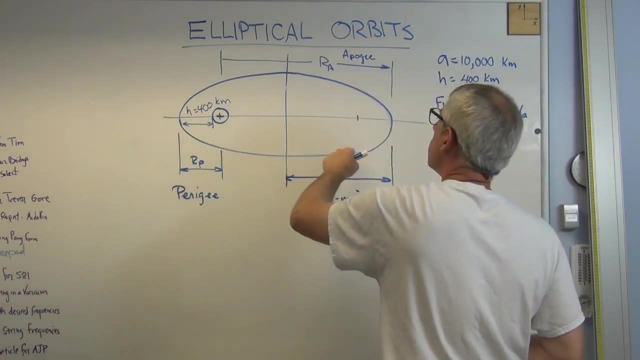 at its closest approach. it's going faster than it would be in a circular room, And that'll orbit. If it wasn't, it would be in a circular orbit. Since it is, it's going to go out farther, trying to, trying and failing to escape the Earth's gravity. 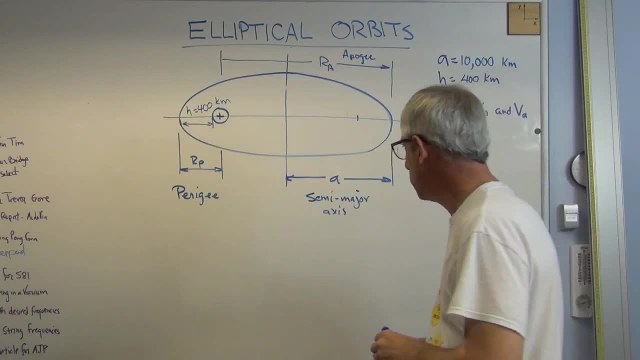 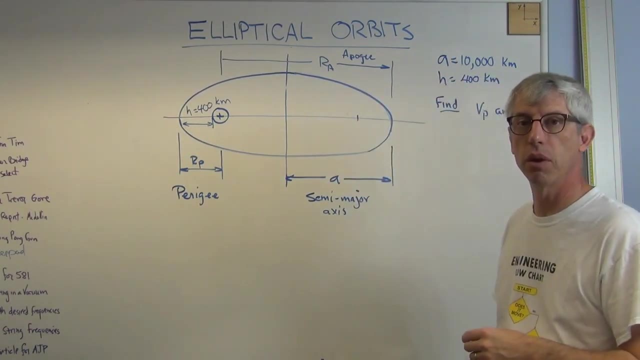 and then it gets drawn back in again. Okay, so let's do this. I'm going to need to erase this picture. I'll get my head out of the way one last time here so you can get one. good look at it, And let's, let's, let's crunch some numbers here. Well, 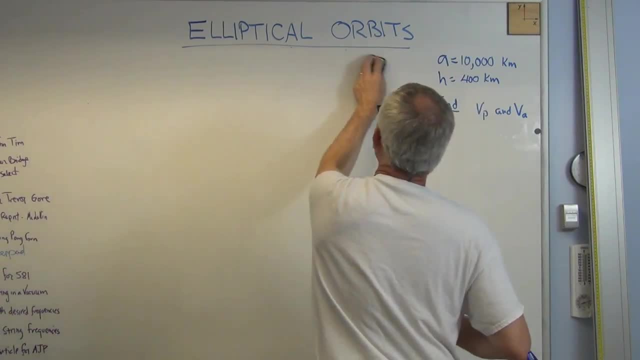 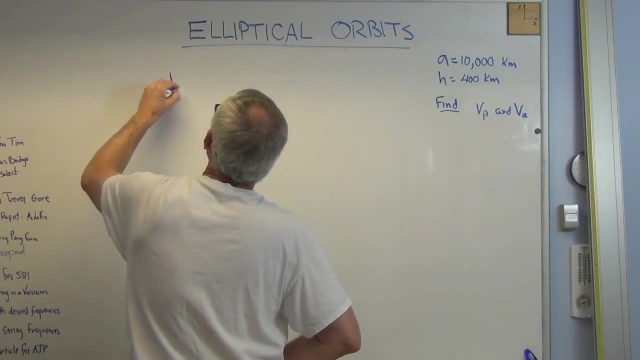 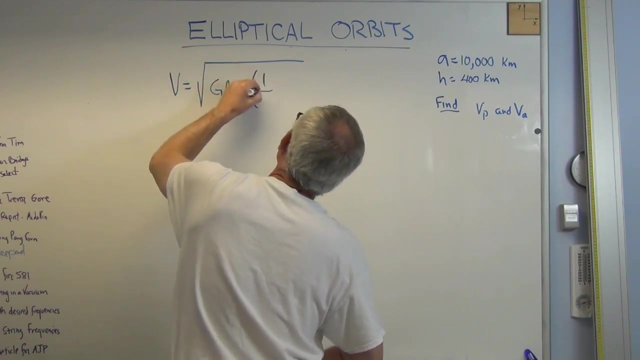 there's there, okay. So the expression for velocity is going to be: v equals the square root of gm of mass. This is mass of the Earth. Oops, that's two over one. I'm sorry I don't. this is one of. 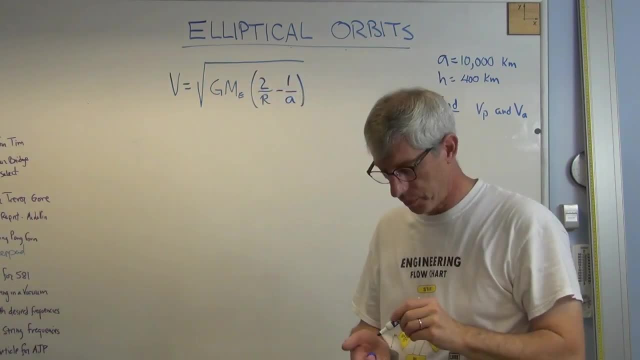 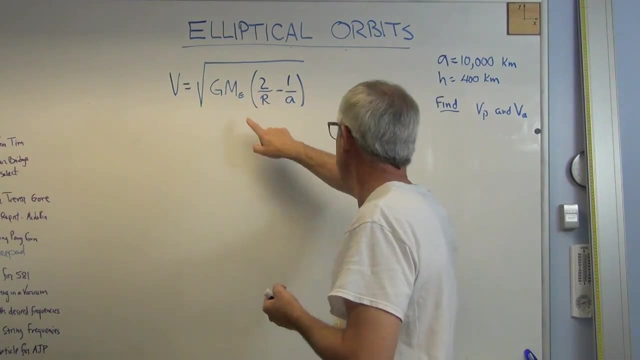 those equations I don't have memorized yet. Okay, so there it is. So you have g, the universal gravitational constant times, the mass of the Earth, which is something from 10 to the 24th. Two over r, where r is the radius from the. 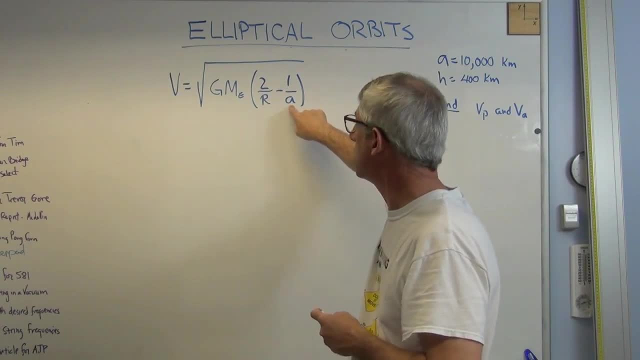 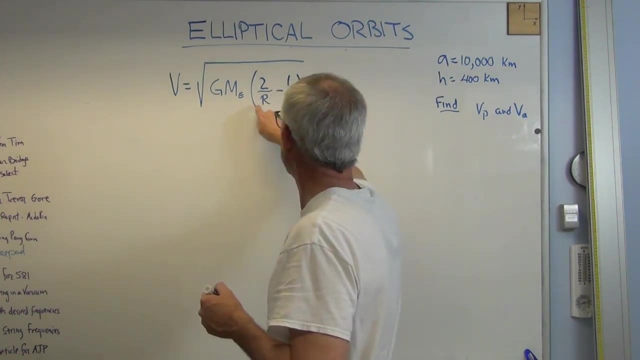 center of the Earth and there's the semi-major axis. Let's see, we already know what that is. It's 10,000 kilometers. We know what these are. I'll write these down in a second. You kind of look these up. What about that one? I need the radius. 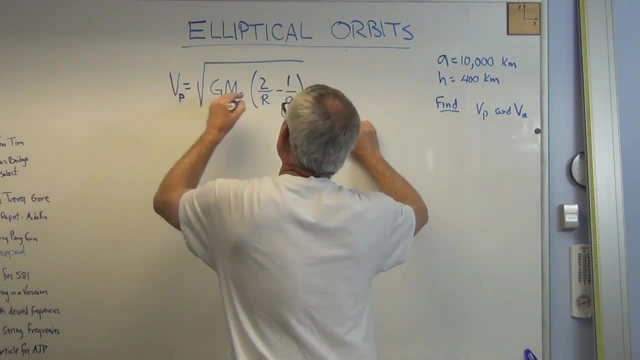 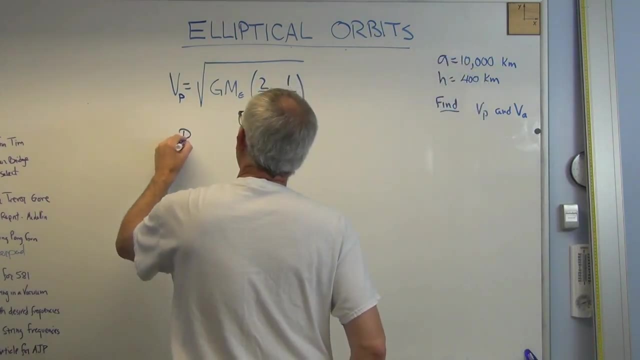 and this. this is going to be. if I want this to be vp, that's going to be rp for the perigee. Well, I don't know what rp is yet. I do know that rp is going to be: let's see h plus the. 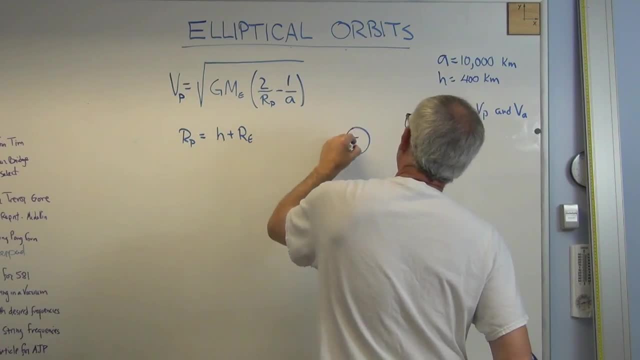 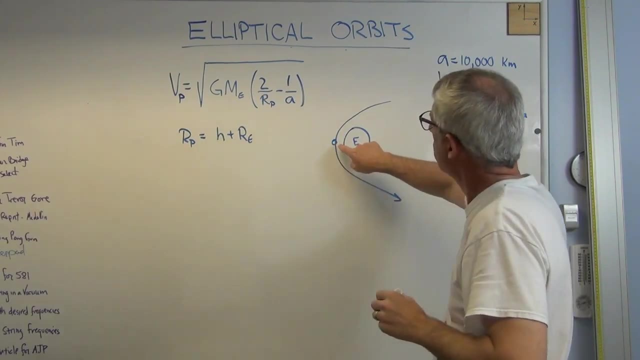 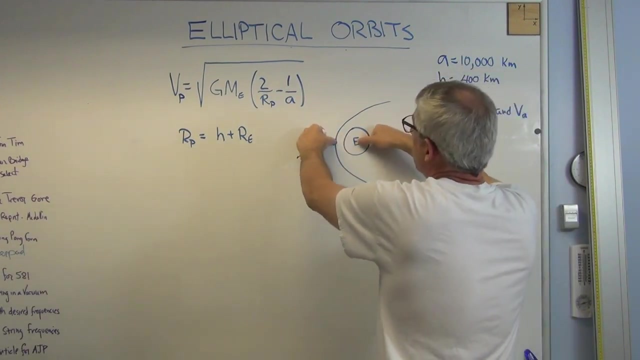 radius of the Earth. okay, because remember what we've got: there's the Earth and this part of the path is this thing comes by. Okay, there's h and there's the radius of the Earth. So the perigee, that radius right there, goes from the center of the Earth to the path of. 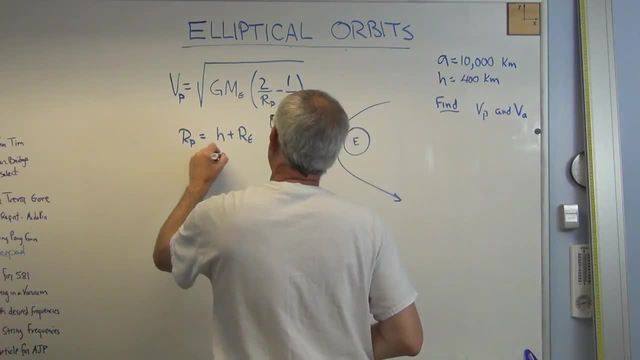 the satellite. So that's going to be…. Okay, So the perigee, that radius goes, from the center of the Earth to the path of the satellite, 400 kilometers plus 6378, right, Oh, where is it? Yeah, 6378 kilometers. 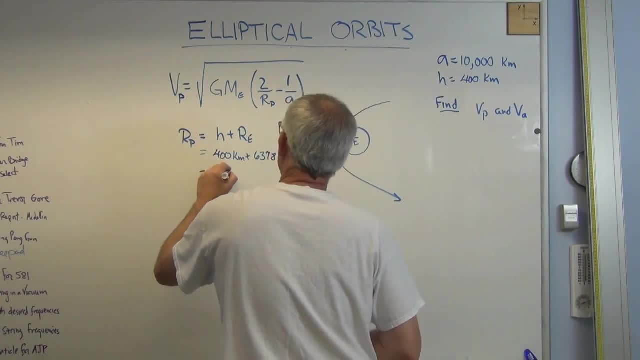 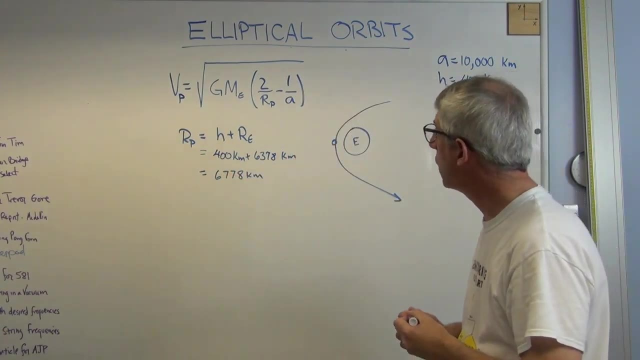 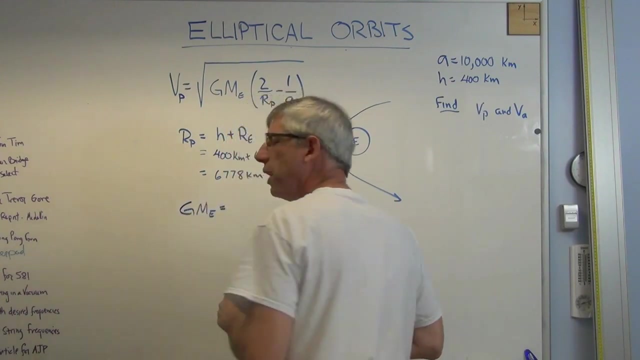 And that's going to be 6778 kilometers. All right, so now we know everything we need to know. If I plug all these numbers in, let me give you one more number, just in case you didn't see the other video, So you don't generally need G by itself, big G. 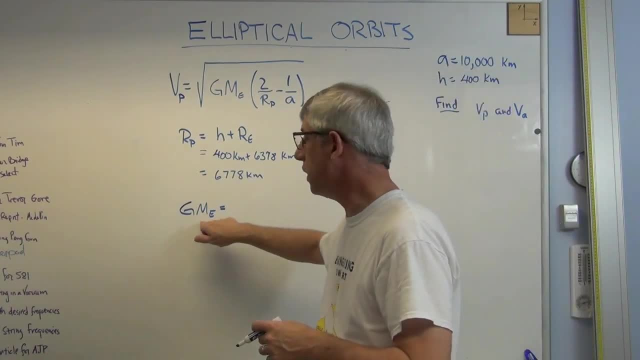 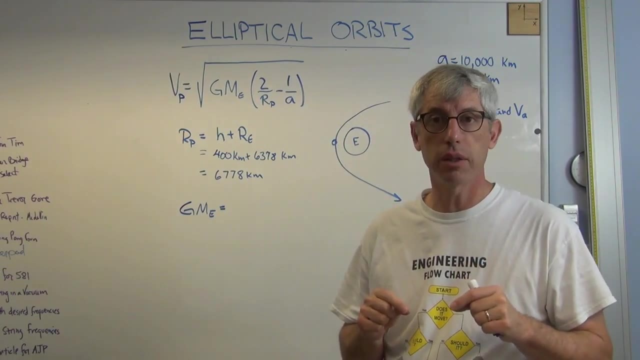 and you don't generally need mass of the Earth by itself, but you generally do need the product of the two. so I'll write those out here in a second. And just a reminder that the universal gravitational constant big G is not the same as little g, the acceleration due to gravity on Earth. 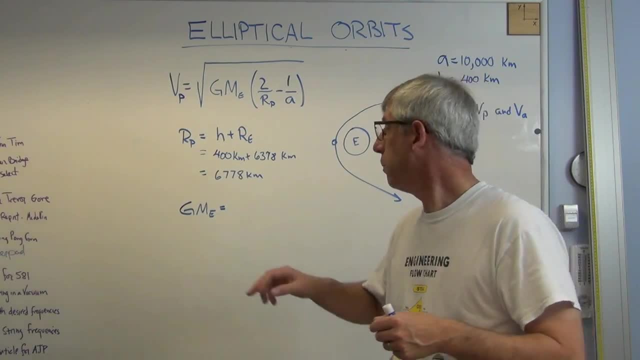 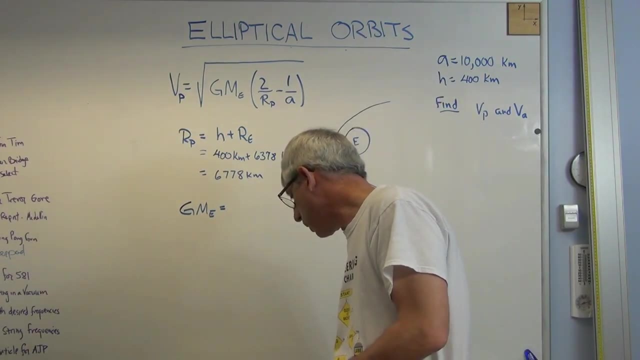 Little g is 9.81 meters per second squared. okay, Big G doesn't change. It's the same everywhere in the universe, as far as we can tell. and it's this crazy number, It's 6.. It's 6,, 7,, 4,, 1 times 10 to the minus 11th. 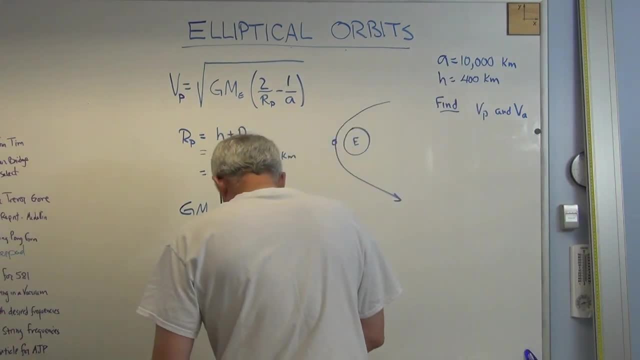 and there's a bunch of units on it, okay, So what we're going to get here is, let's see, 3.9859 times 10 to the 14th meters, cubed, second squared. okay, And this is not an intuitive number. 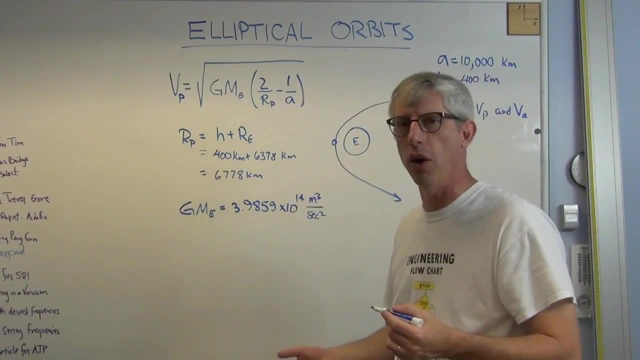 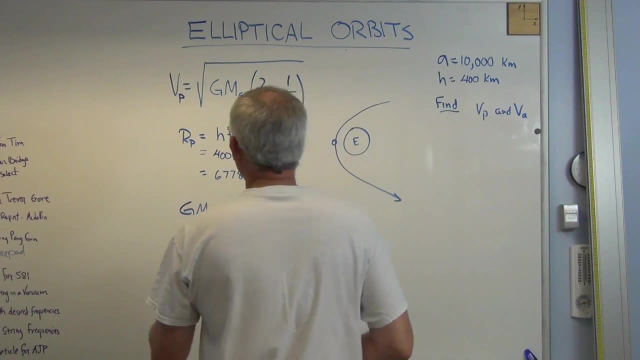 You would never look at this problem and go: oh gee, golly, it's obviously that. No, You have to look this one up in Calculator. All right, so there you go. How far can I go down here? Okay, so if I work all that out, 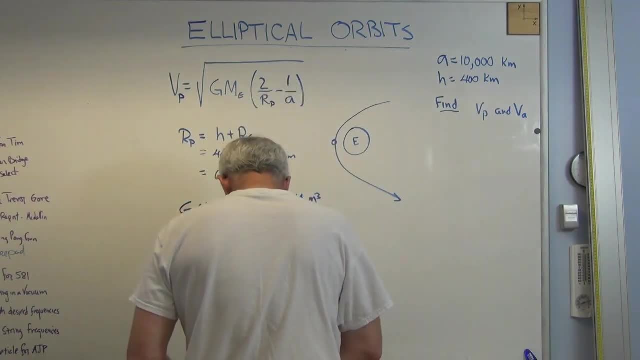 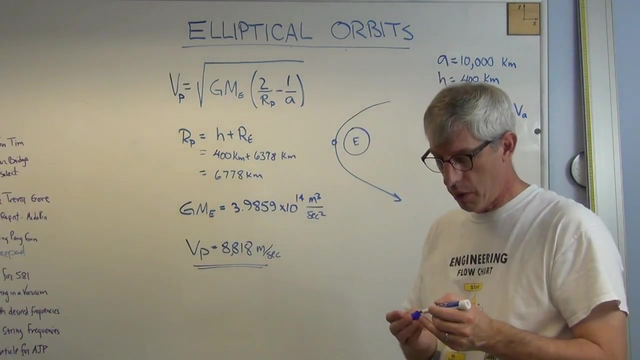 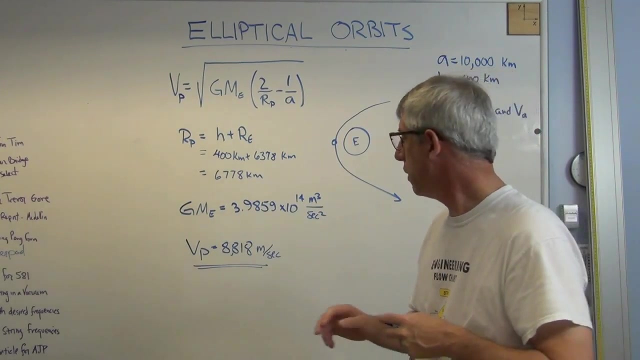 what I'm going to find out is that Vp is 8,818 meters per second. okay, That's the velocity at the closest approach. Now the velocity if the satellite was in a circular, if the satellite was in a circular orbit, is about 7,700,. okay, 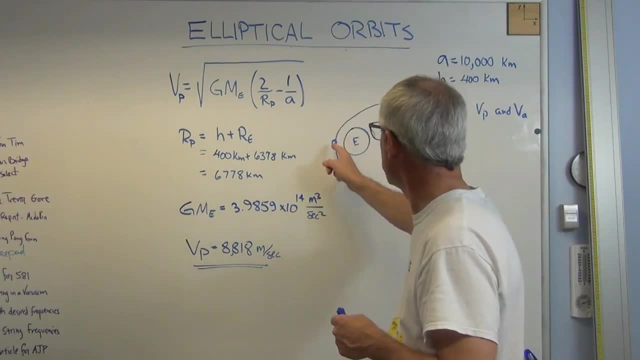 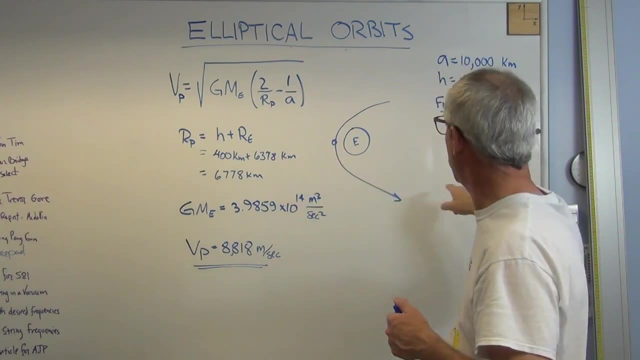 So this is significantly higher than that and that's why it has the energy to move away from the Earth and then get pulled back. It's turning excess kinetic energy into potential energy to go way out here and then trading it back again as it comes back around the other side of the orbit. 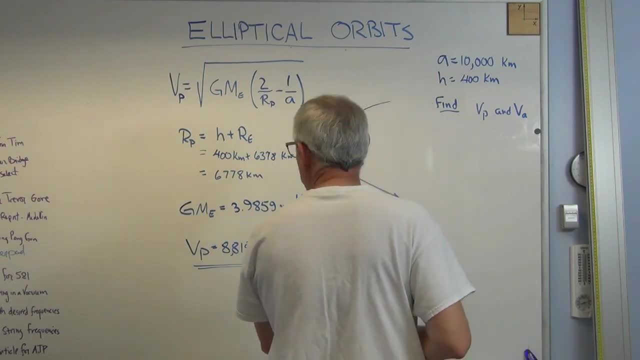 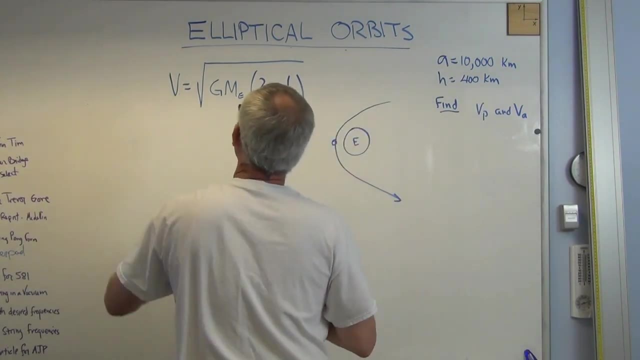 Okay, so that worked. What do we get if we use Va or I use A? if we can find Va, Let's check. Let's change that. We want to know the velocity at the apogee and then we need to know the radius at the apogee. 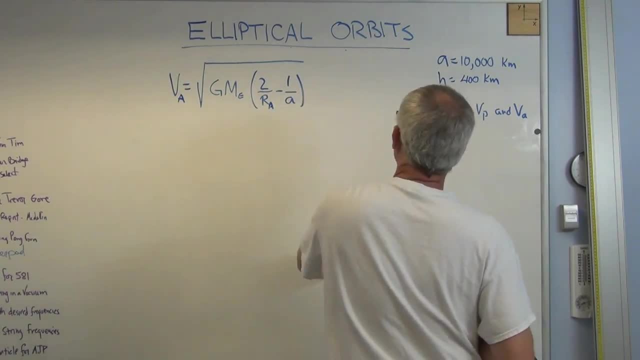 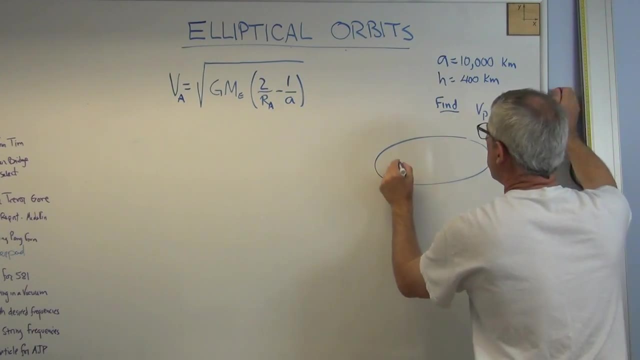 So this isn't right anymore. okay, Draw this in a slightly different way here, a little smaller, maybe That's not too bad. Okay, that's Ra. So I'm trying to find. let's see, we're going that direction. 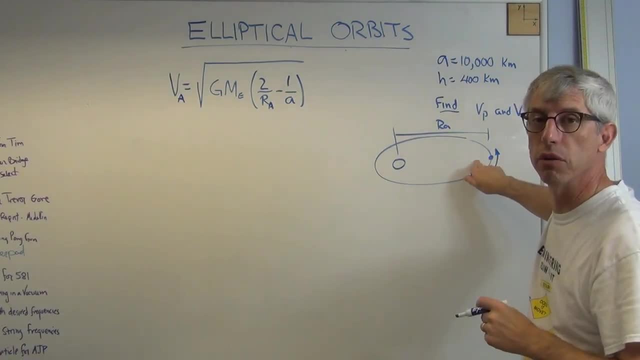 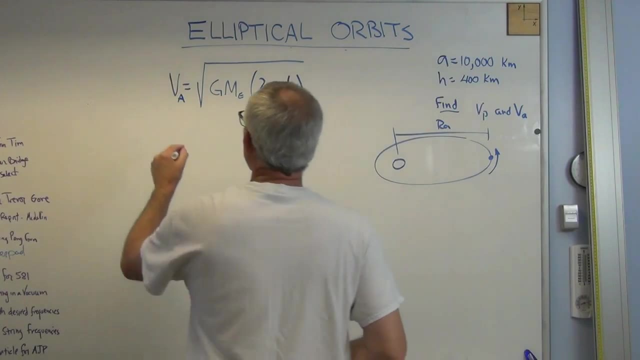 I'm trying to find V. It's at its farthest excursion from the Earth. Now it should be less than that low Earth orbit velocity. It should be less than 7,700 meters a second. I'll actually write all this out, I guess, just so you can see it. 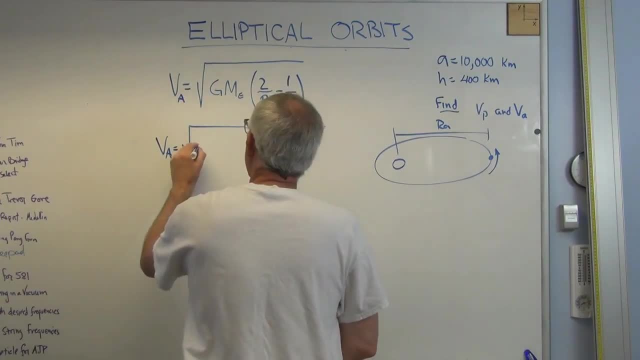 Okay, what is this? 39859.. 14 meters cubed, second, squared 1 over. oh, we don't know, Ra, do we? How are we going to do that? Well, let's see, Ra, let's take what we do know, okay. 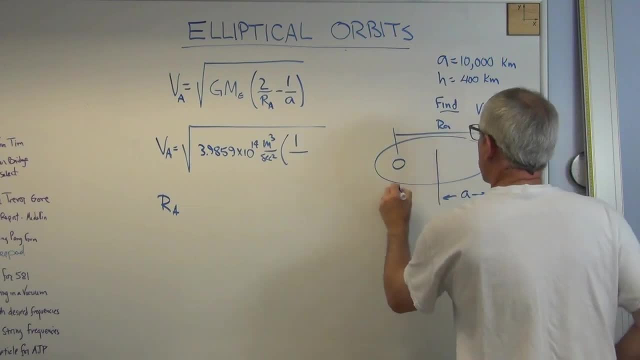 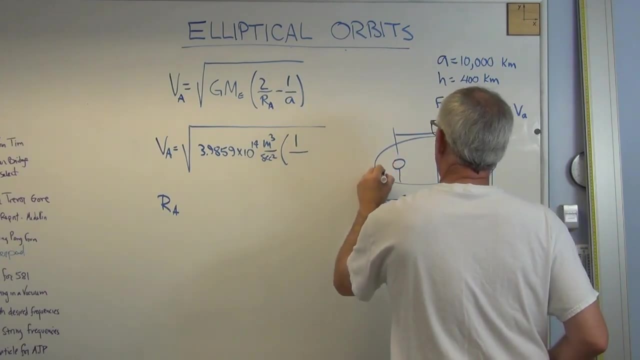 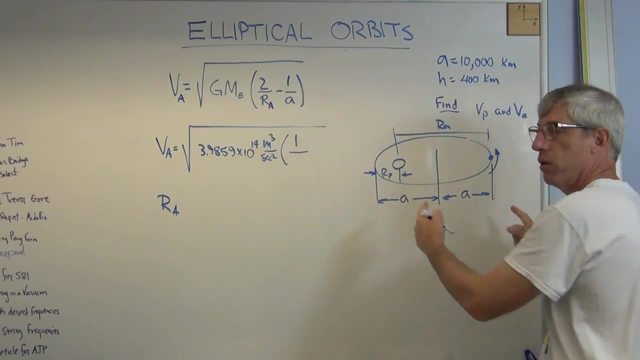 We know that's a and we know that's a. okay, So, and that's Rp, right there. okay, So Ra must be 2a, that's the width of the ellipse minus Rp. Well, that's not so bad. 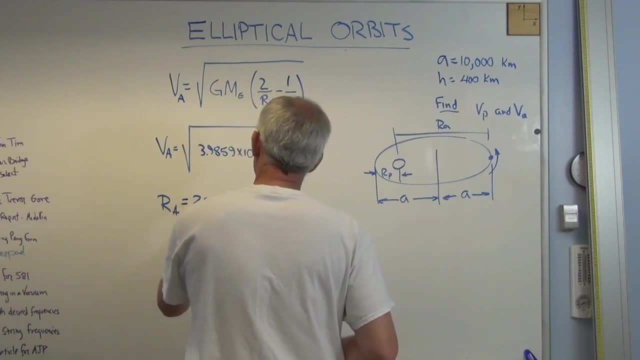 And we know what Rp is. So if you work that out, you get 1322.2.. So I've got 1322 times 10 to the 7th meters or 10 to the- let's see- 4th kilometers, if you want to do it in kilometers. 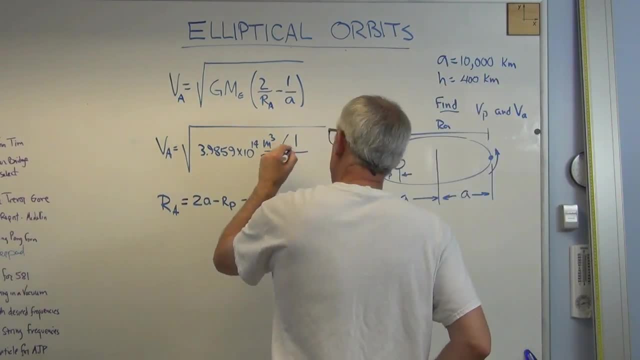 By the way, you have to do this all in base units, So this is all going to have to be in meters. Uh-oh, going to run out of room, let me, I'm going to have to get rid of this. 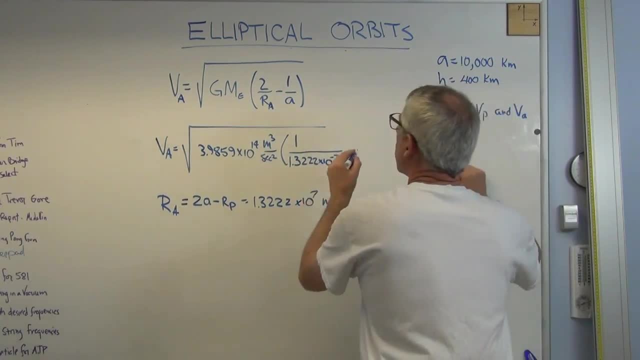 I need a bigger board, don't I? And this is 10,000 kilometers, 10,000,. I'm going to actually write all this out, just so you can see what it looks like there. These numbers get big, okay.